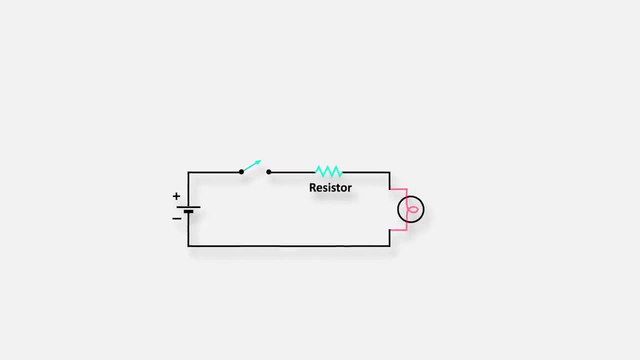 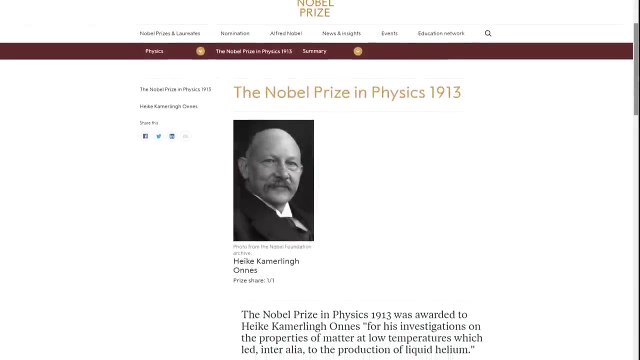 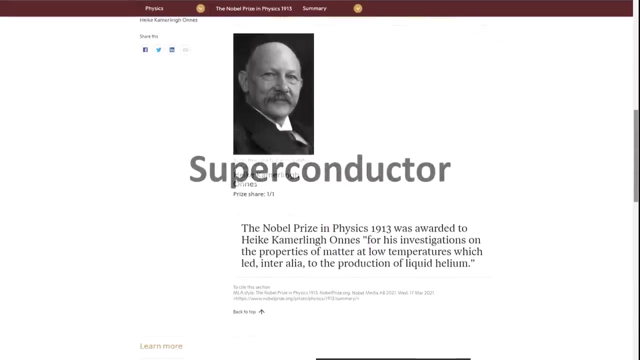 which meant no energy loss. This was highly unusual, because normally at least some energy is lost in the process of electrical flow through materials. Recognizing the importance of this phenomenon, he called this new state of matter a superconductor. Onnes received the 1913 Nobel Prize in Physics for this discovery. 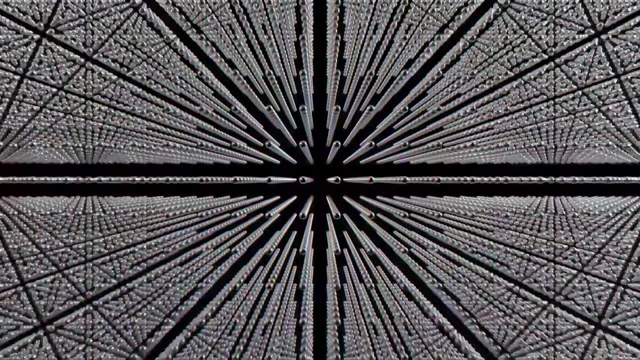 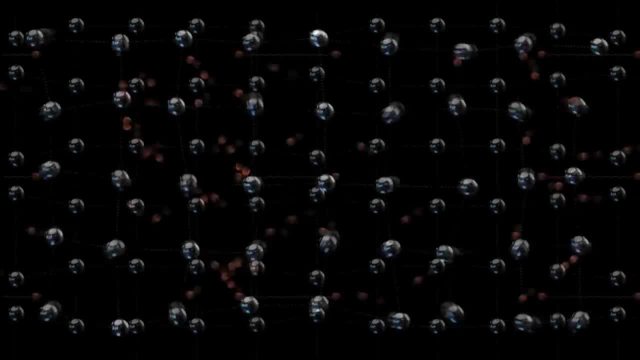 Under ordinary conditions, when electricity flows through a material, there's always a resistance. There's no resistance to this flow because electrons bump into atoms, causing some energy loss in the process, But somehow, as if by magic, in this new state of superconductivity. 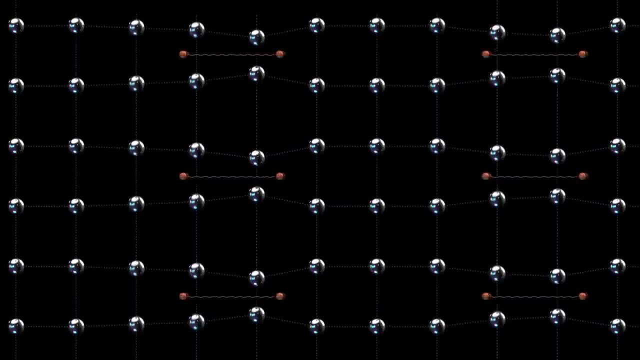 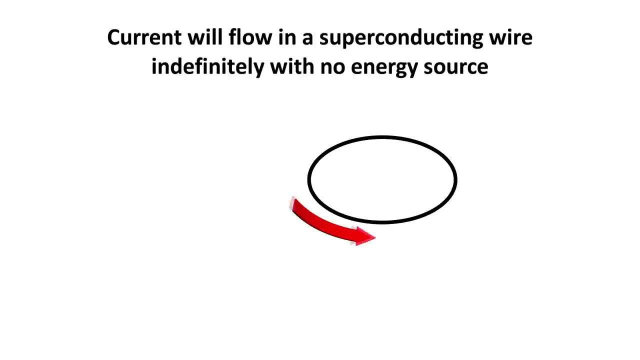 the electrons flowed right through the material as if there weren't any atoms in their way. In fact, this material is such that if you put a current in a superconducting wire, in a loop, that current will continue to flow virtually forever with no added voltage or energy source. 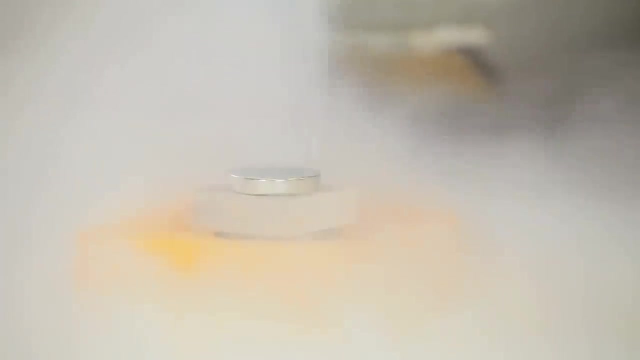 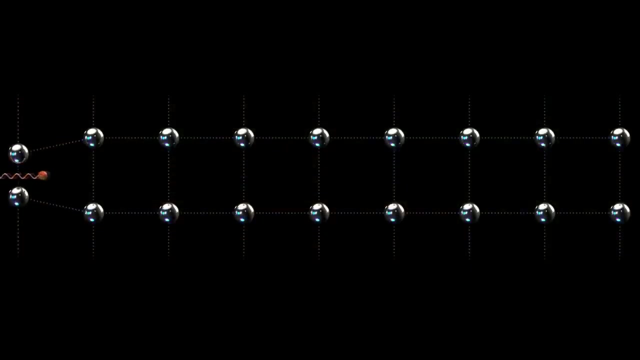 And superconductors have another seemingly unique feature in that they expel magnetic fields. So if you put a magnet over a superconductor, the magnet will levitate. How is this possible? How can any material carry current perfectly with no energy loss? To answer this question, we have to dive deep into the subatomic realm. 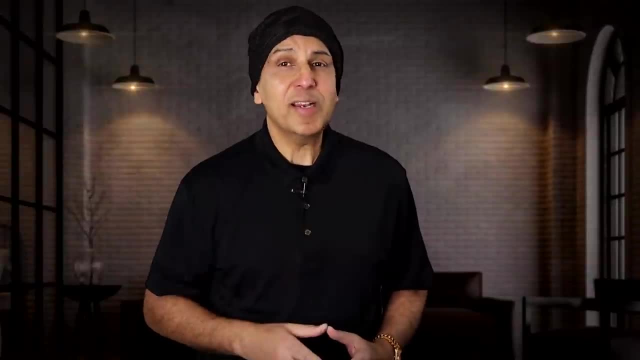 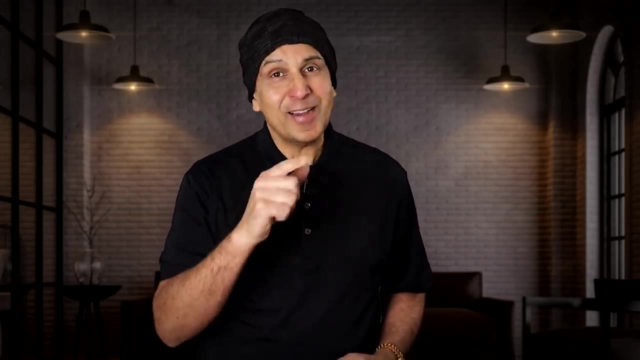 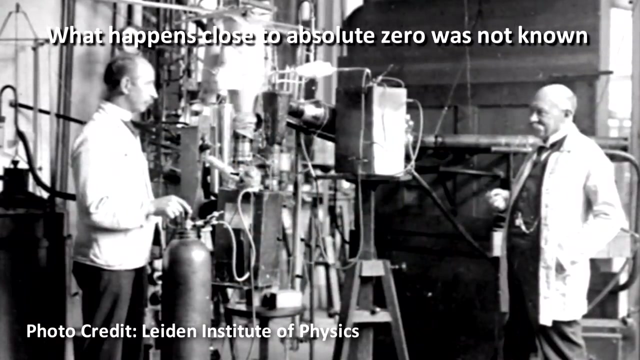 which means we have to invoke quantum mechanics. What is superconductivity? Why is it so special And how does quantum mechanics explain it? The answers are coming up right now, While the idea of materials reaching a low resistance at very cold temperatures was 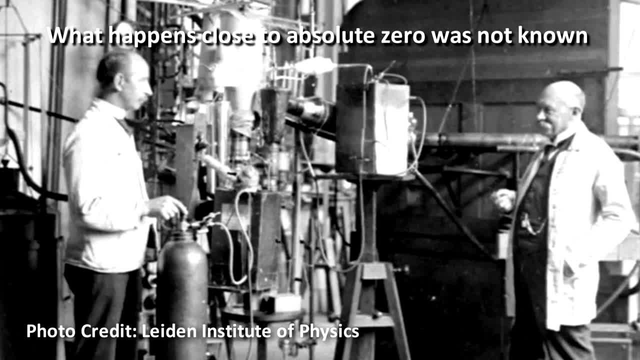 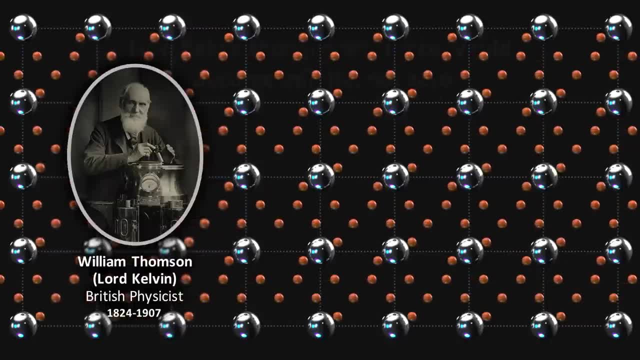 rather well accepted. the question was: what happens at or close to absolute zero? Lord Kelvin thought that electrons would completely stop and thus the resistance would become infinite. So when it was first discovered that a material's electrical resistance can become zero at very low temperatures, this was unexpected In 1911,. 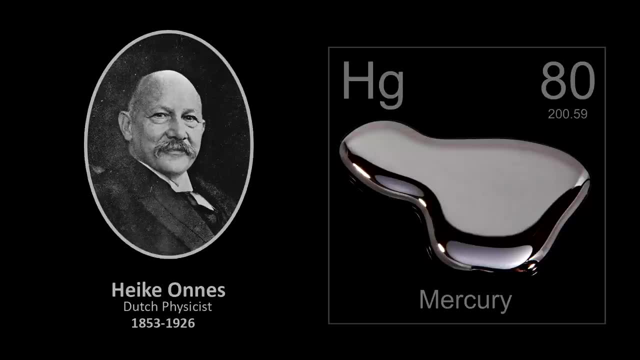 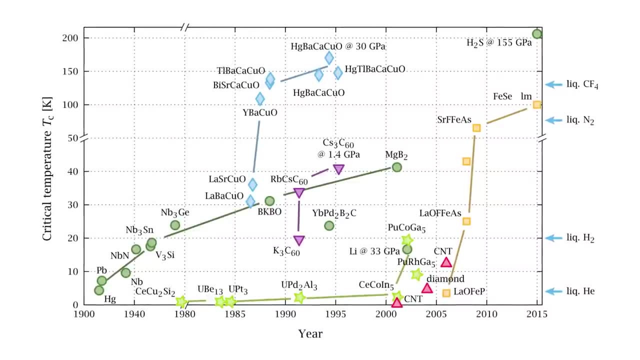 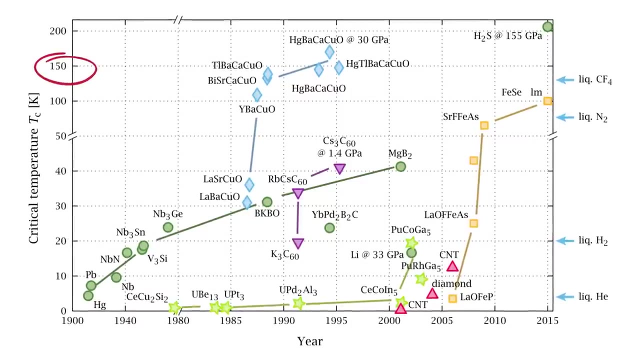 he was the first to discover this in mercury and found it to be superconducting at 4.2 degrees kelvin. Later it was found that other materials and alloys can be superconducting at much higher temperatures. Typical temperatures, however, are still pretty cold, usually lower than 150. 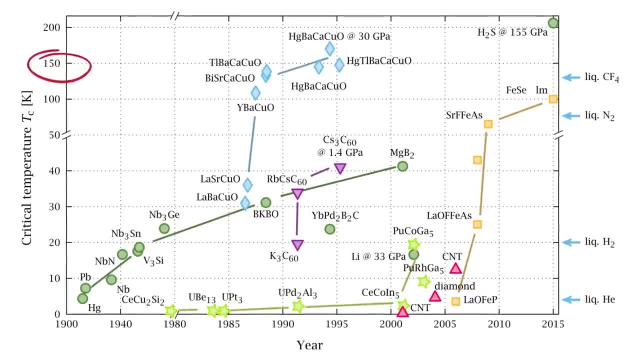 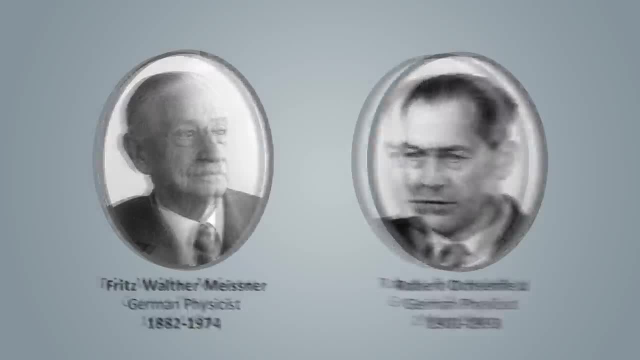 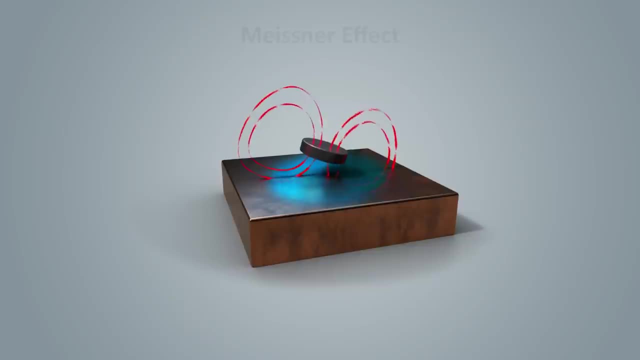 degrees kelvin or negative 123 degrees celsius. The next big discovery was made in 1933 by Walther Meissner and Robert Ochsenfeld. They found that when a metal is cooled, while in a small magnetic field, the flux is spontaneously excluded, as 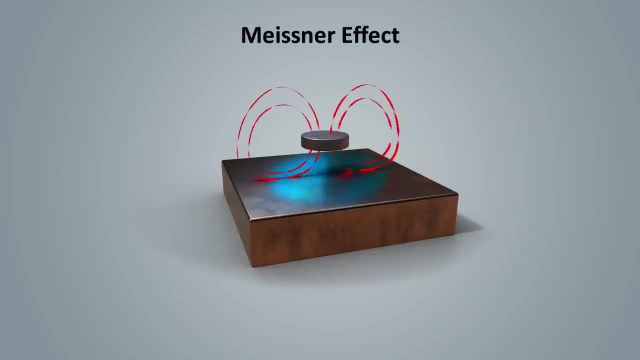 the metal becomes superconducting. This is known as the Meissner effect. Normally, matter allows magnetic fields to pass through it. However, a property of superconductivity is that superconducting materials expel magnetic flux fields, In other words, 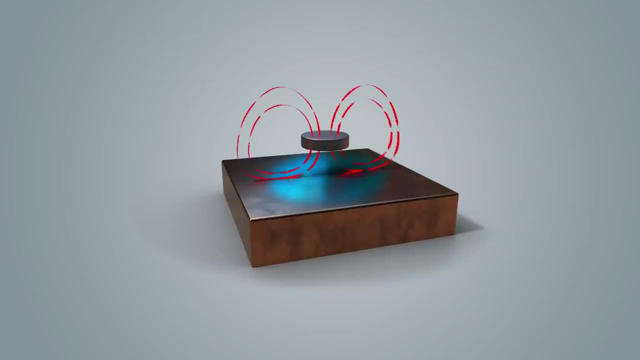 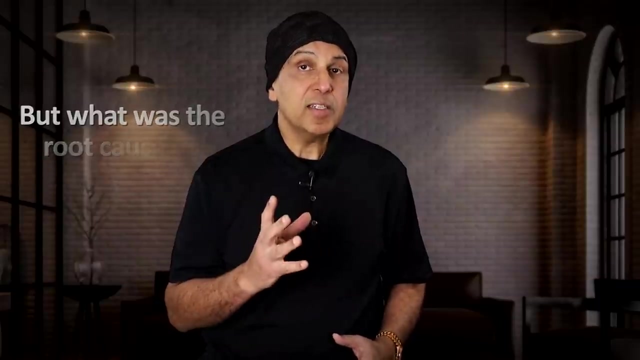 magnetic fields cannot pass through it. So the magnetic field of the magnet lifts the material in order for the flux to flow to the opposite pole, which causes levitation. Even after this discovery, it was still not known what exactly was the cause of superconductivity. It was not until 46 years after the discovery by Onas that 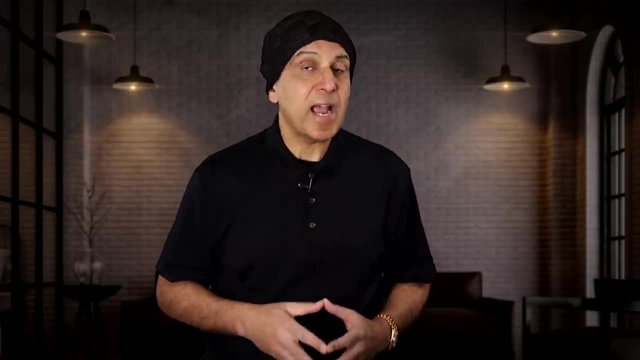 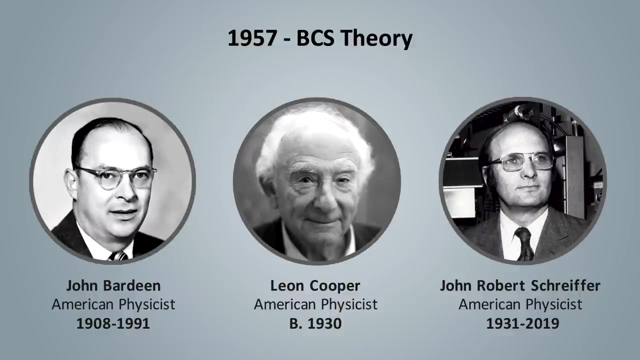 we got the first real microscopic theory to describe what is actually going on. In 1957, John Bardeen, Leon Cooper and John Robert Shriver proposed what is now called the BCS theory. in their honor It earned them the 1972 Nobel Prize in Physics. So what did they do? 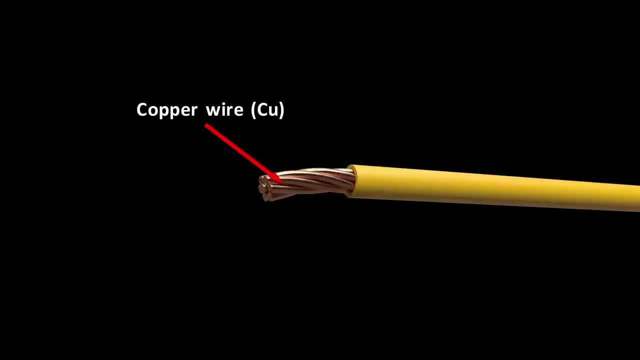 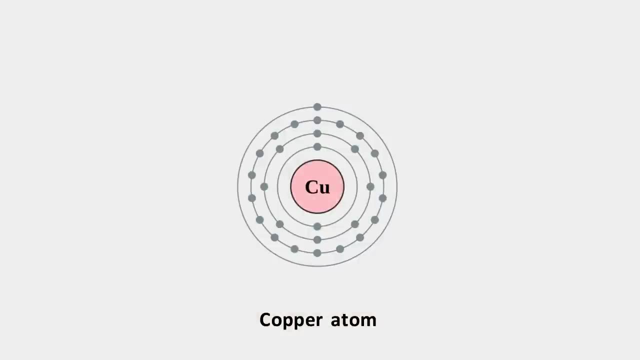 To understand how electrons can flow with no resistance in superconductors, we first need to understand what causes resistance in the first place. Inside of a metal, the outermost electrons in the valence shell being furthest away from the nucleus, are so free to move around. 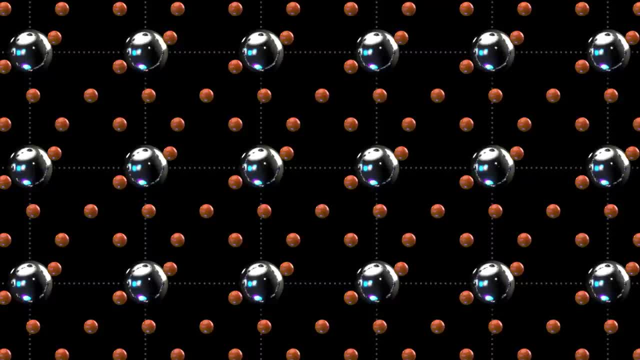 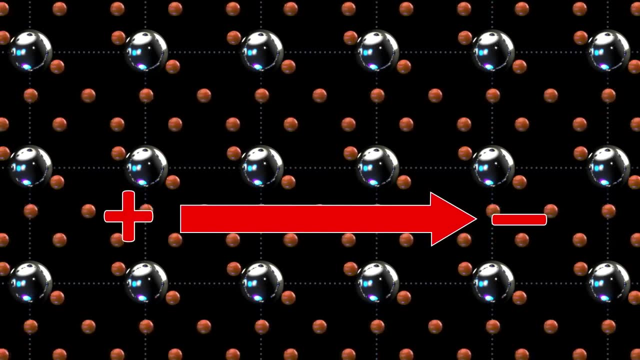 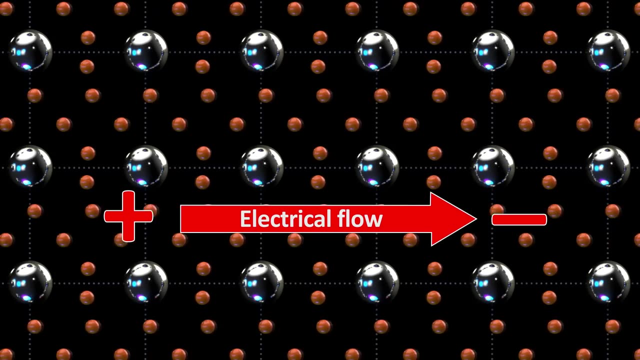 that a sample of metal can be treated as a bunch of atoms surrounded by a sea of electrons. The electrons can flow in a liquid-like manner. If we add electricity to one side of the metal, the metal accepts these new electrons easily and it pushes out some electrons on the other side to 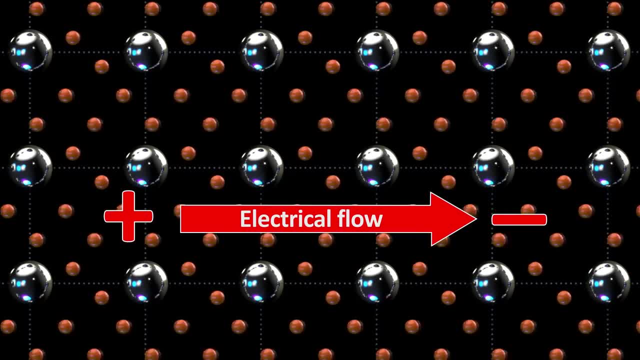 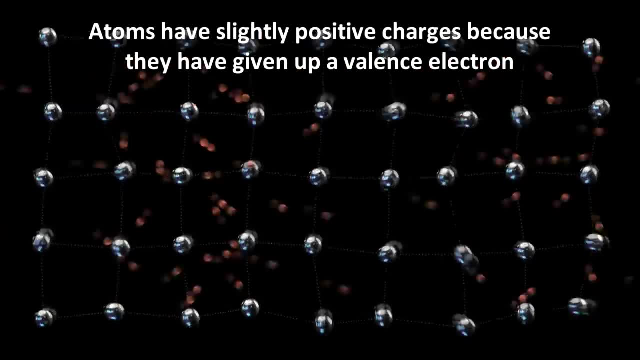 make room. We interpret this flow as a current of electricity, But the electrons don't flow perfectly. As electrons travel through the material, the atoms, which now have slightly positive charges because they've given up an electron in their outer shell, are in the way. 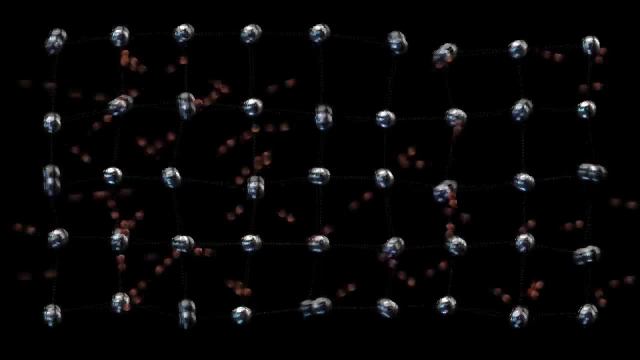 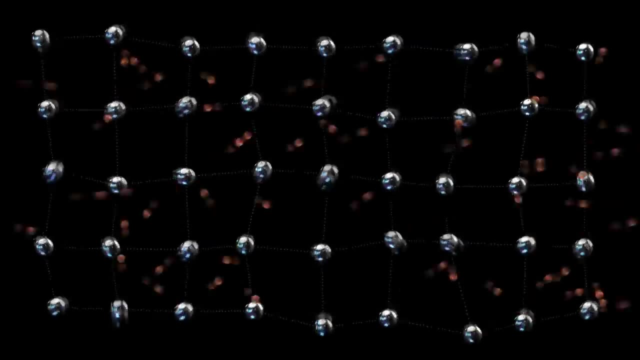 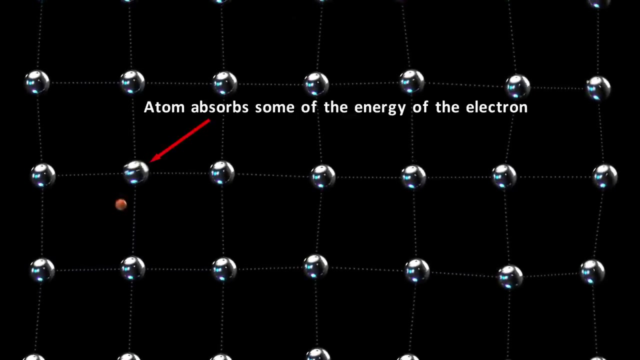 If the atoms were perfectly still, the electrons would have an easier way to sneak through the material, But this is usually not the case. The atoms vibrate or there are imperfections in the lattice. The electrons collide with the atoms that may be vibrating. This causes the electrons to scatter and it ends up giving up some of its 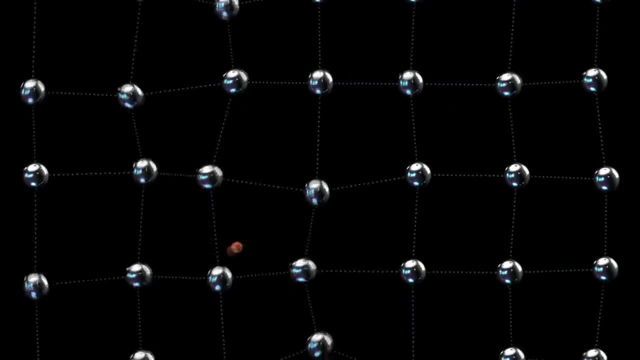 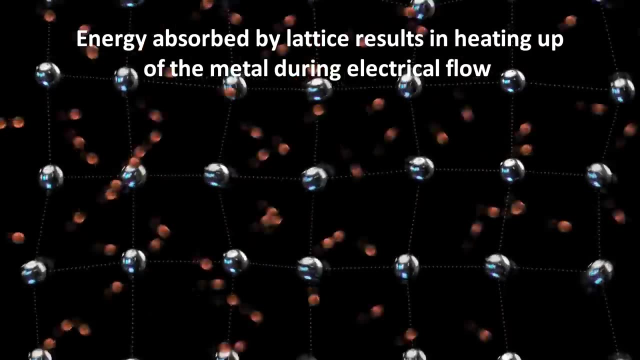 energy to the atom, causing it to vibrate a little bit more. This added vibration causes the whole lattice to vibrate a bit more. This higher vibration results in heating up of the metal. So this is how energy is lost. due to resistance, Under normal conditions, even the best conductors. 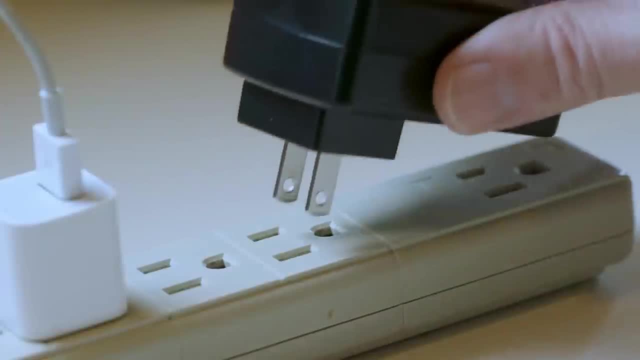 have some resistance to electrons. This is how energy is lost due to resistance. Under normal conditions, even the best conductors have some resistance to electrons. You might even feel this heat loss sometimes if you put your hand over the power cord of your devices As the temperature. 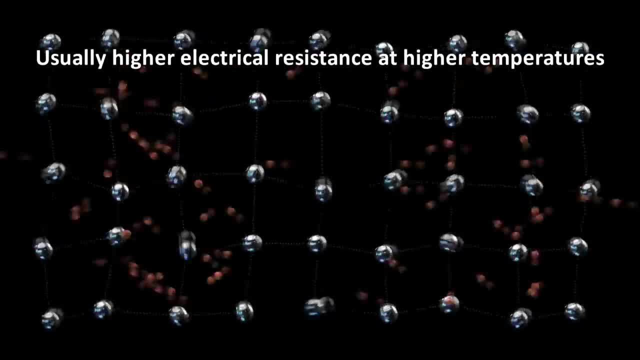 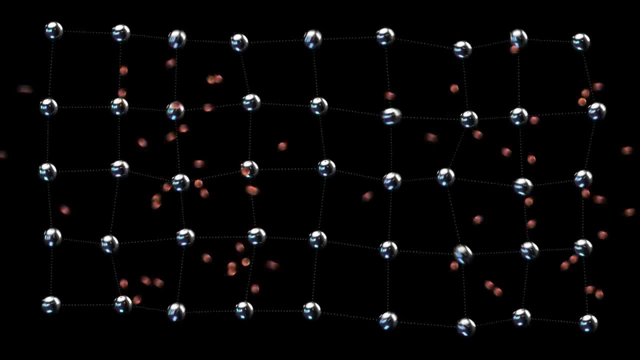 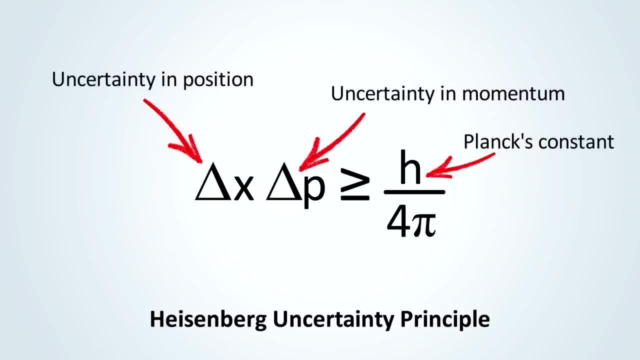 rises, the atoms vibrate more strongly, causing more energetic collisions and higher resistance. The vibration which causes the electrons to scatter can be reduced by reducing the temperature of the metal, But the nature of quantum mechanics, specifically the uncertainty principle, is such that there will always be a little bit of motion. This is called zero-point energy. There's 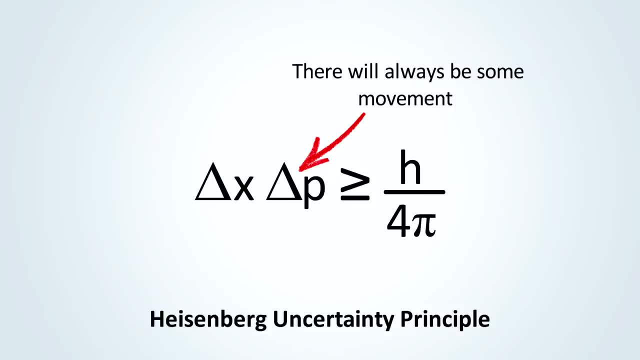 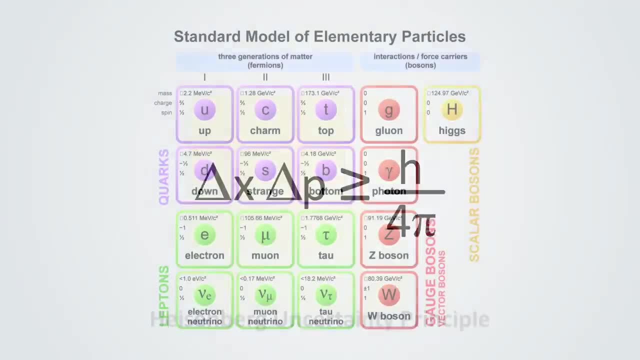 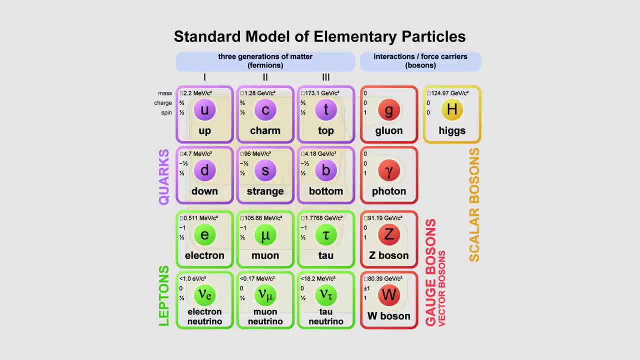 always some motion, because the uncertainty principle states loosely that no quantum object can have precise values for its position and momentum at the same time. So now that you understand what causes resistance in the first place, let's look at how this resistance goes away completely. But to understand this, 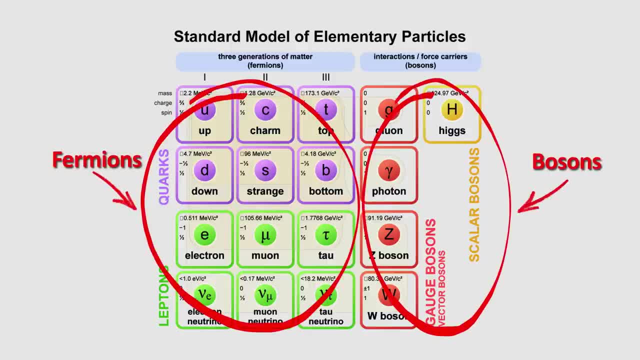 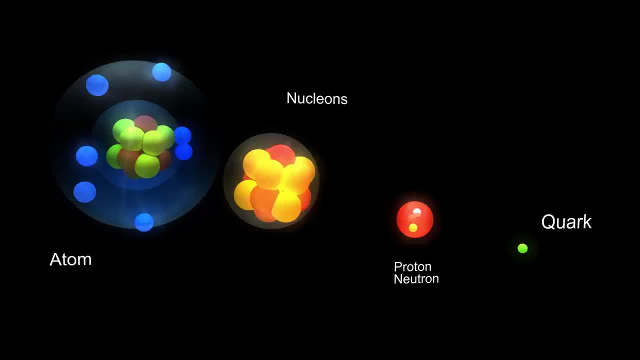 I have to introduce you to two terminologies in particles called fermions and bosons. You know that matter is composed of particles. You've heard of protons, neutrons and electrons. Each of these particles has a certain property related to momentum. 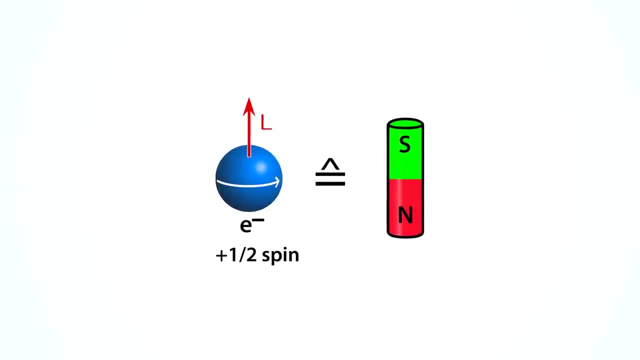 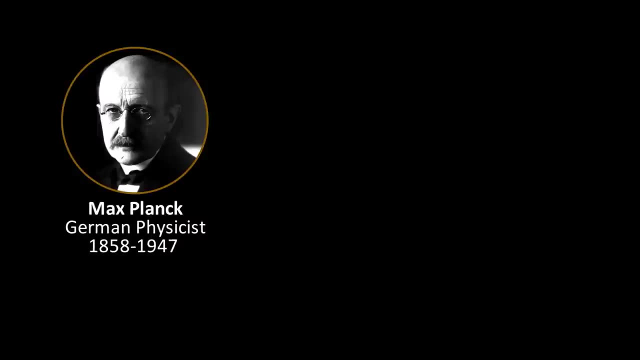 called spin. Note that spin doesn't mean a physical spinning, but is called spin because electrons act like tiny bar magnets with an angular momentum. These values of spin are multiples of Planck's constant, one of the fundamental constants of the universe, which relates the energy that a photon can carry to its frequency. The values of spin are either: 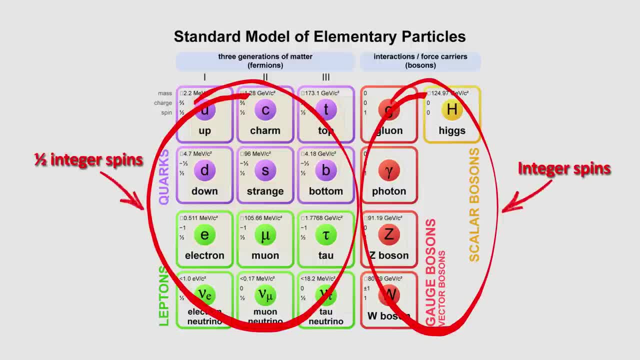 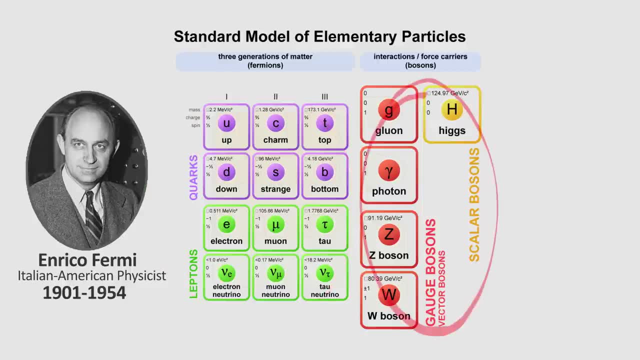 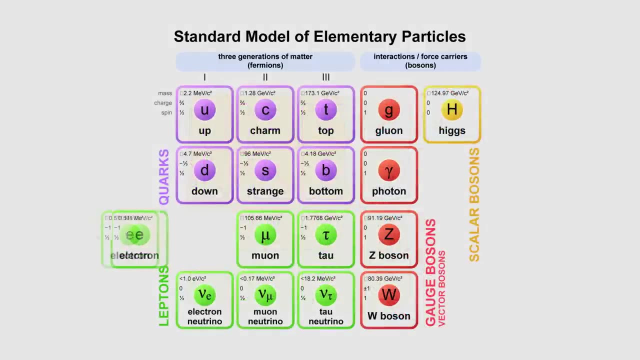 integer multiples of Planck's constant or half integer multiples. A particle with a half integer spin is called a fermion, named after Italian scientist Enrico Fermi. A particle that has an integer spin is called a boson, named after Indian scientist Satyendra Bose. An electron can have a spin of plus one. 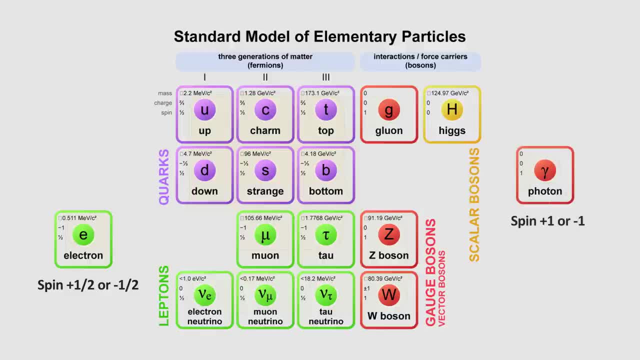 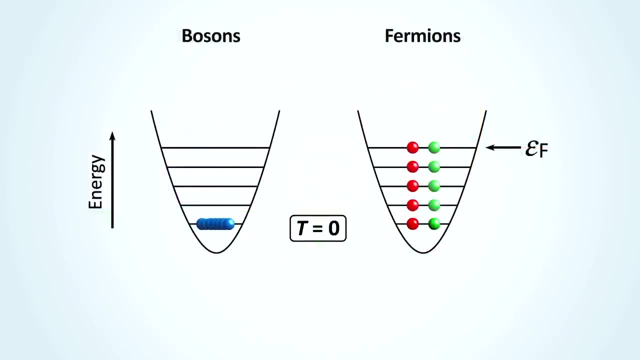 half or minus one half, so it is a fermion. A photon can have a spin of plus one or minus one, so it is a boson. Fermions and bosons behave differently at the subatomic level. It turns out that while any number of identical bosons can 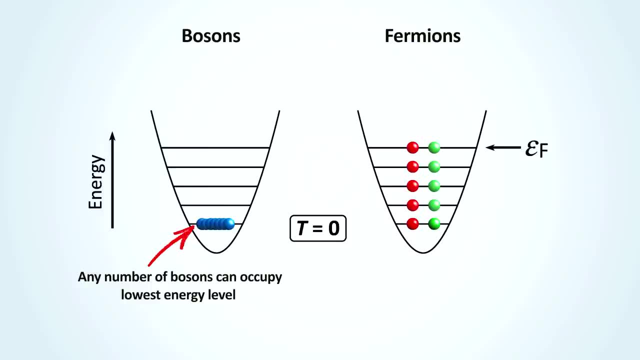 occupy the same energy level in a quantum system. this is not the case for fermions. Two or more identical fermions cannot occupy the same energy level in a quantum system. This is called the Pauli exclusion principle. This is why you can only have two electrons in. 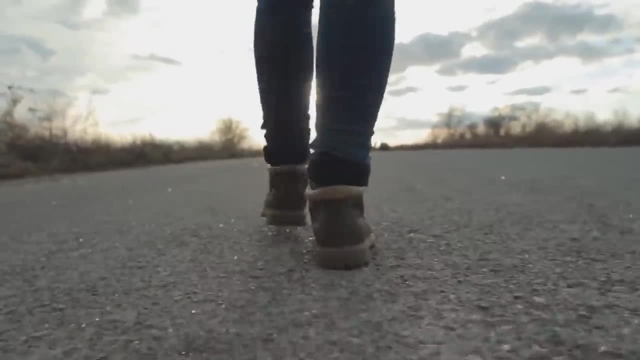 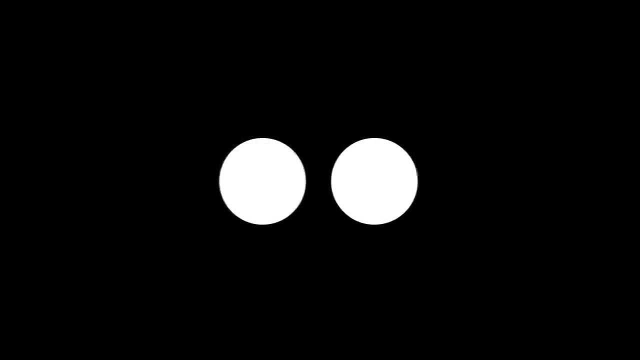 any given orbital of an atom. This is why solid objects can't pass through each other, and you don't pass right through the floor or through a wall. The electrons of the atoms on your feet cannot occupy the orbitals of the electrons on your feet. 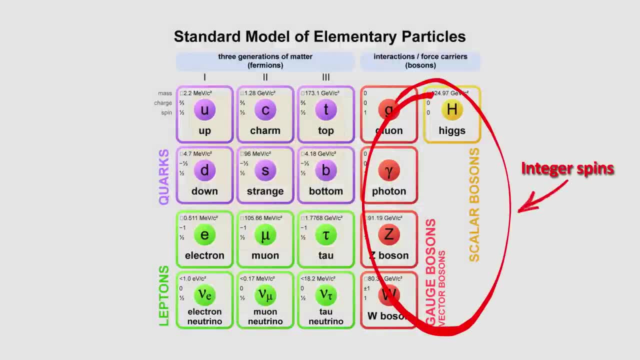 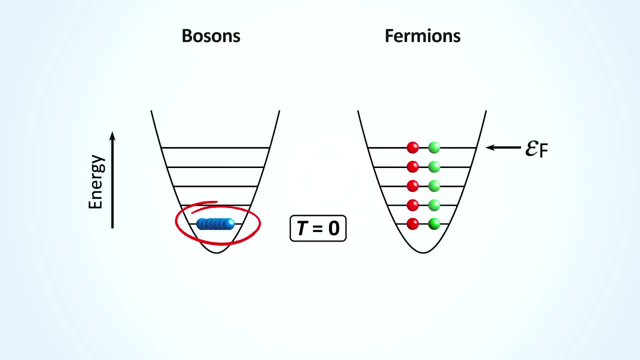 However, bosons are a different kind of beast. They don't have this restriction. In fact, it appears that they like to pack together when there are a bunch of them around, especially at low temperatures, As an electron moves through a conductor. 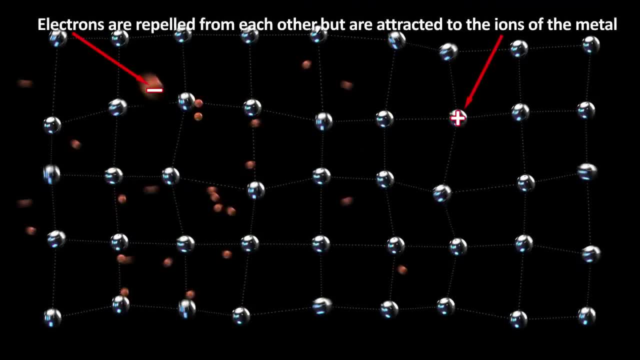 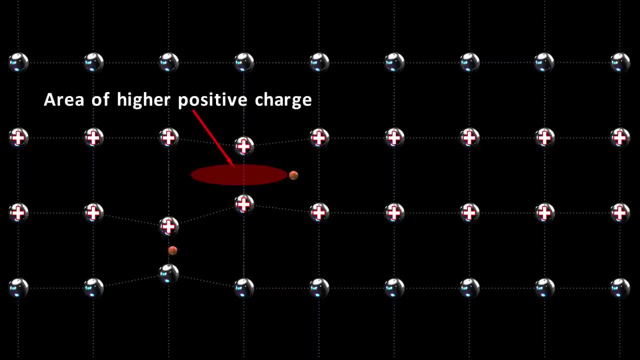 it is repelled from other electrons due to their mutual negative charge, But it also attracts the positive ions that make up the rigid lattice of the metal. This attraction distorts the ion lattice, moving the ions slightly towards the electron, increasing the positive charge density of the 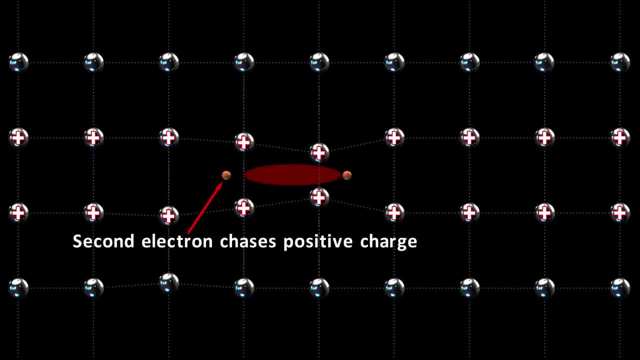 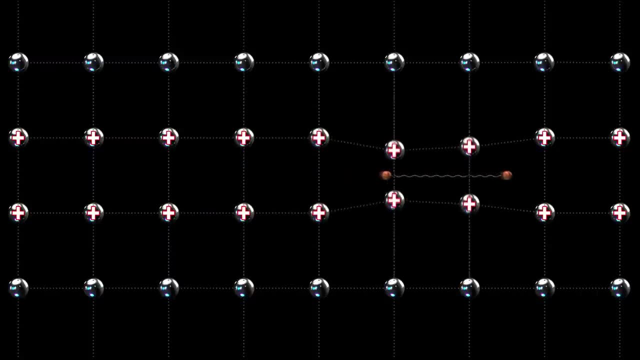 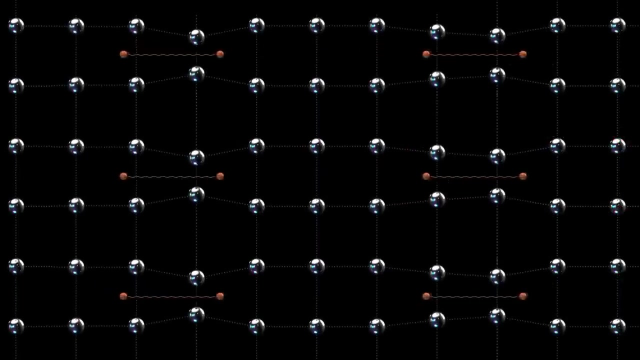 lattice in the vicinity. This positive charge density attracts other electrons At long distances. this attraction between electrons due to the displaced ions can overcome the electron's repulsion and cause them to join. Two electrons, when joined together in this way, are called a cooper pair, And the positively charged region of the atomic lattice is part. 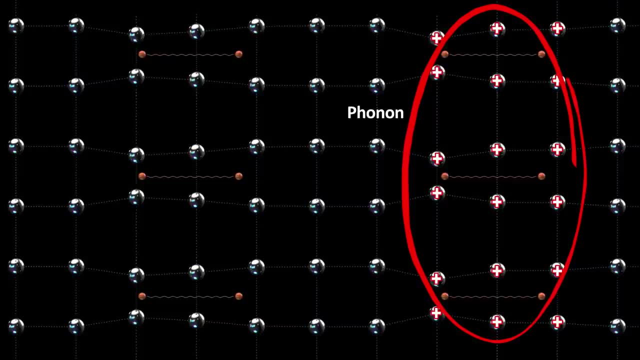 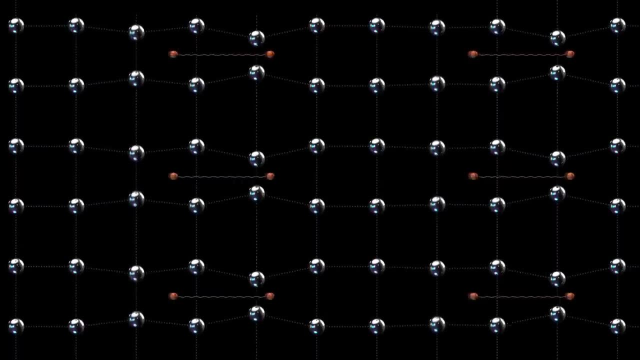 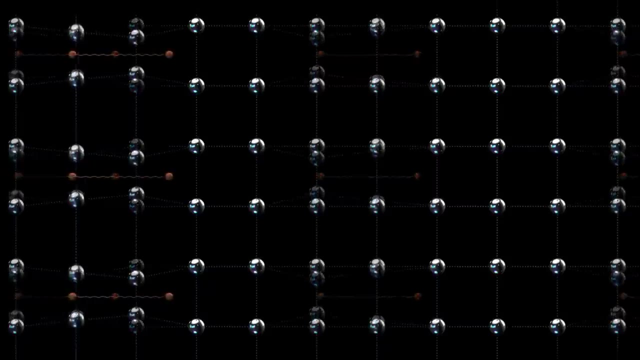 of what is called a phonon. A collective motion of multiple ions with the same frequency are called phonons. Phonons are important for conducting heat and sound through solids, but for our purposes they are important in understanding superconductivity. If the temperature of the material is low enough, the cooper pair remains together. 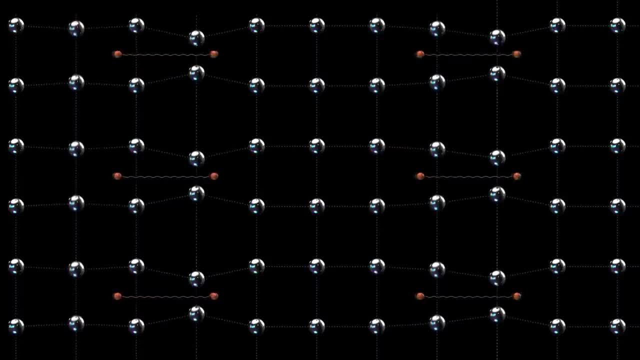 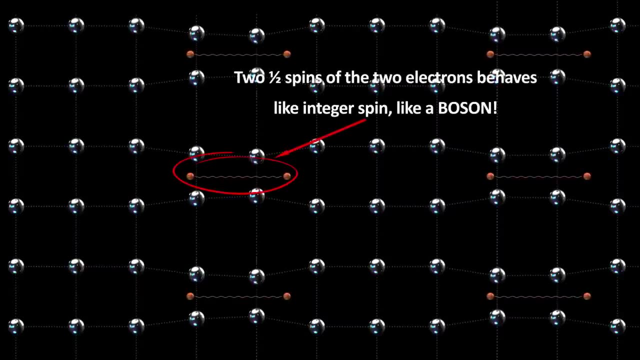 because it does not have enough energy to break apart. This pair can then be treated as a single particle. When two electrons come together in this way, their half-spins interact in such a way that together they form an integer spin. In other words, they start behaving like bosons instead of fermions. They are no longer subject to the 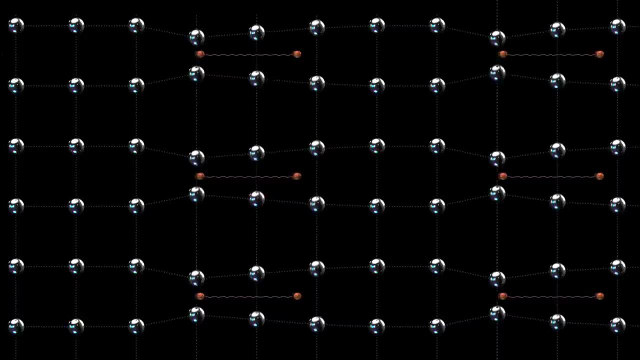 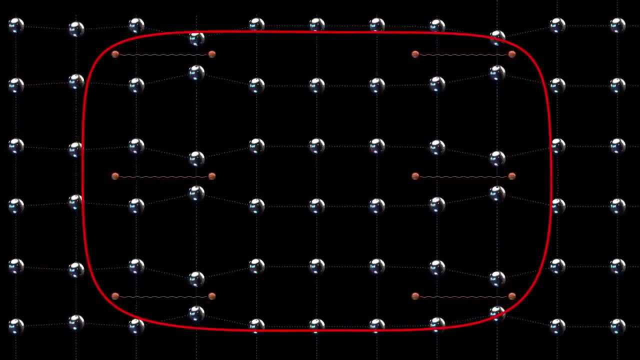 Pauli exclusion principle. What happens now is that, since an arbitrary many bosons can fit into the same low energy state, the collection of cooper pairs starts acting like one entity or unit. This state when a bunch of bosons cooled to low temperatures occupy the lowest quantum. 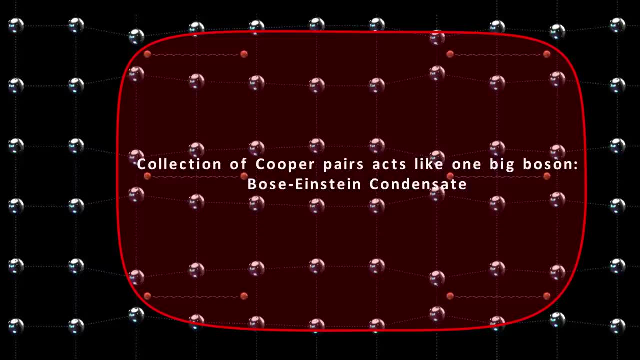 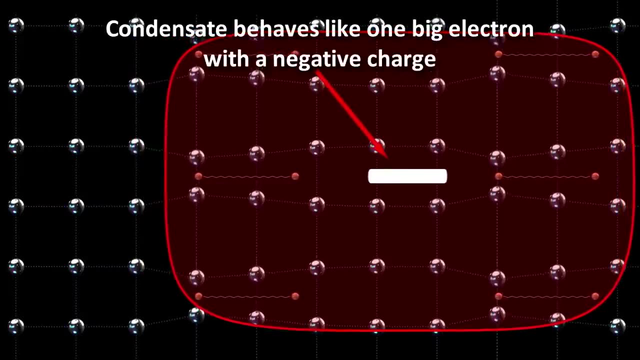 ground state is called a Bose-Einstein condensate. They act like one bosonic electron, all at the same low energy state, And it is negatively charged because it is made up of electrons that are negatively charged. So this means it can conduct electricity. 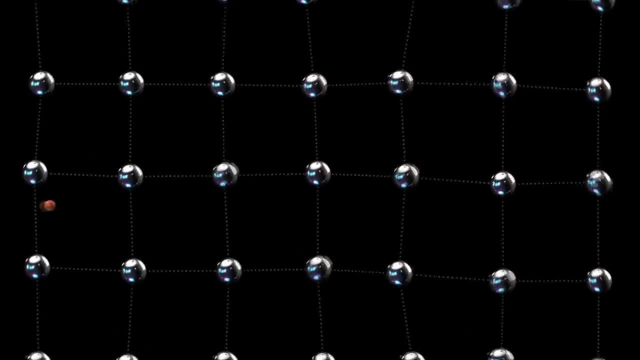 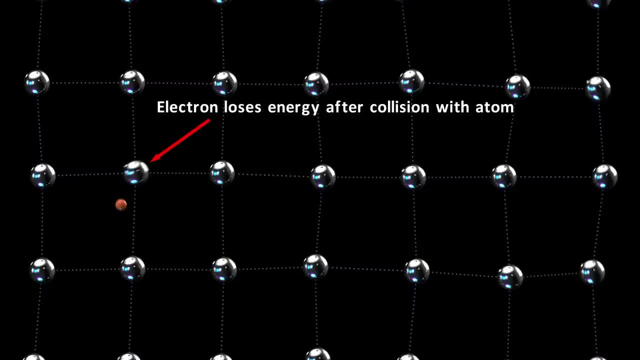 Normally when an electron collides with an atom and scatters, it loses some energy by going to a lower energy state than before it collided. This energy is lost to the lattice of the metal. But with cooper pairs there is no way to solve this problem. 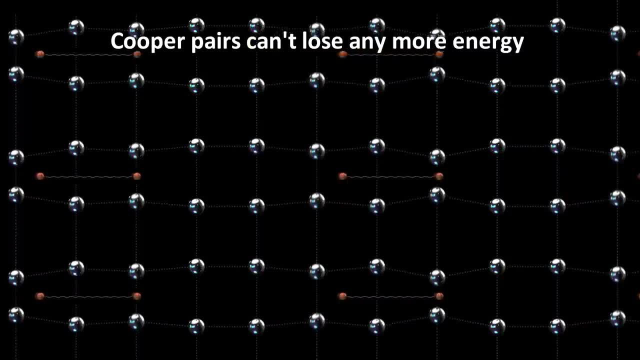 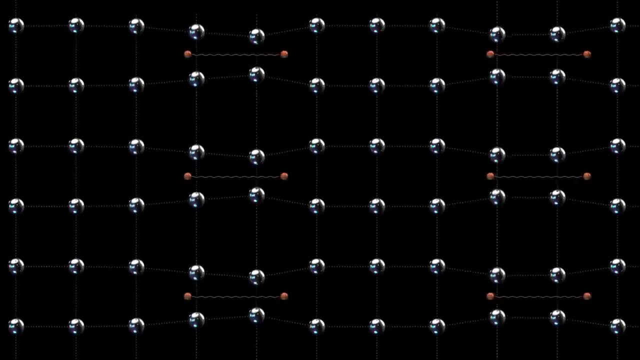 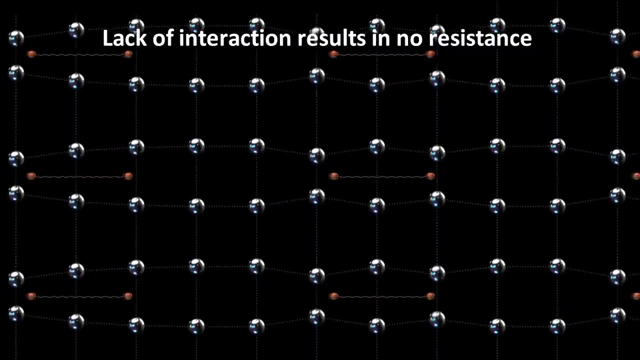 There is no lower energy state for it to go to. There is no quantum state that these bosons can occupy that is lower because they are already at their lowest energy state. So no energy is lost because they can't lose any more energy. The lack of interaction of the cooper pairs with the atoms. 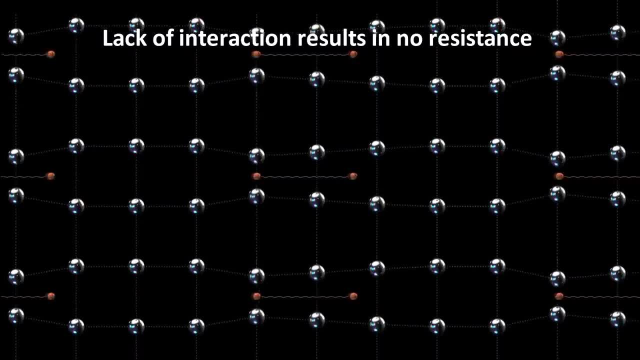 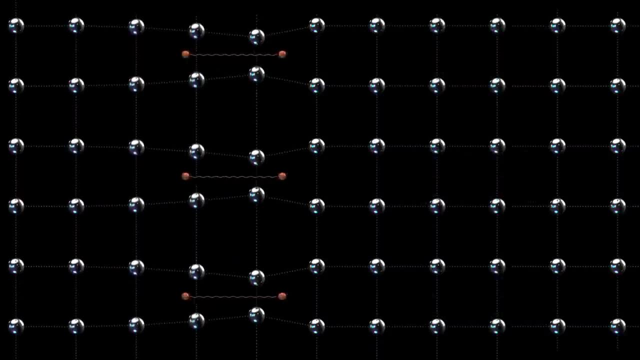 effectively results in no resistance to the flow of electrons, and the material becomes a superconductor. The interaction of the electrons in a cooper pairing is very weak, so it typically only happens at very low temperatures. This is why it is called a Bose-Einstein condensate. 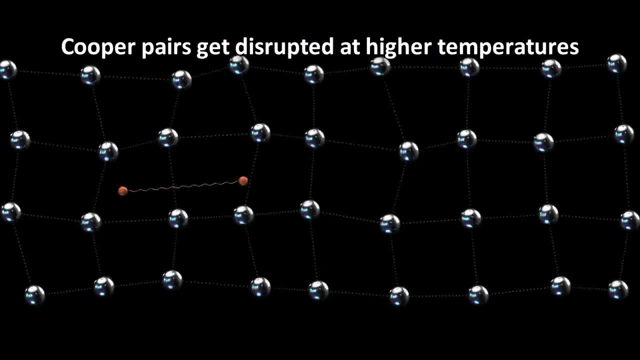 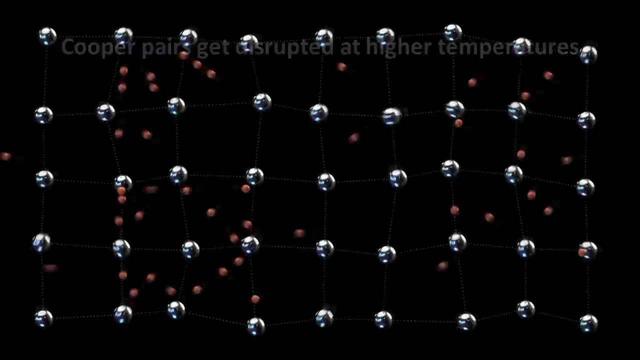 As the temperature gets above the critical temperature, the cooper pairs get disrupted because there is enough energy to break them up, And so superconductivity is lost. It is the formation of cooper pairs through their interaction with the phonons of the material that are the cause. 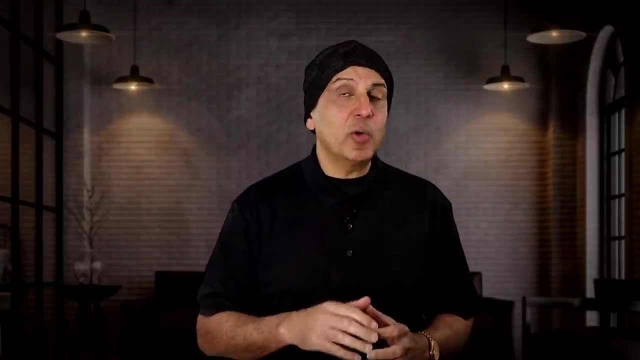 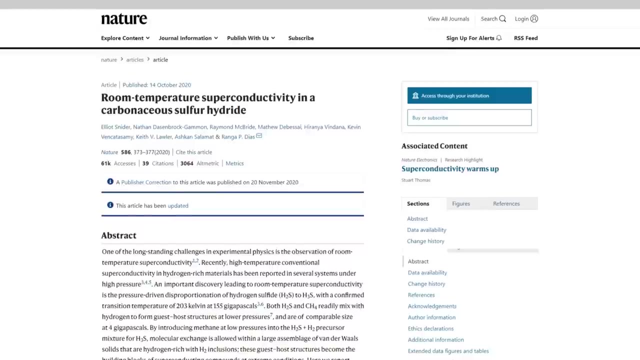 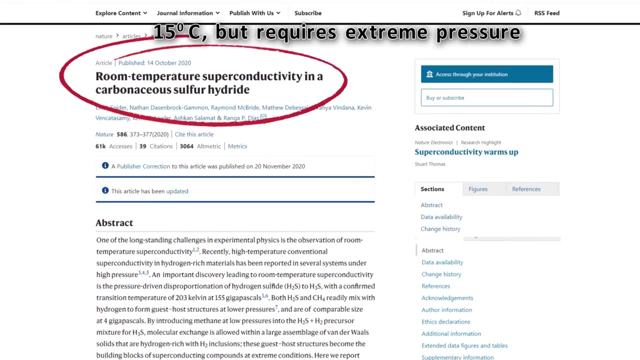 of superconductivity. You should know that the mechanism shown in this video is the conventional understanding of how cooper pairs form, but there are likely other mechanisms that we have yet to understand. A lot of research is going into this field. today, In 2020, the first room temperature superconductor was synthesized. It is a carbonaceous. 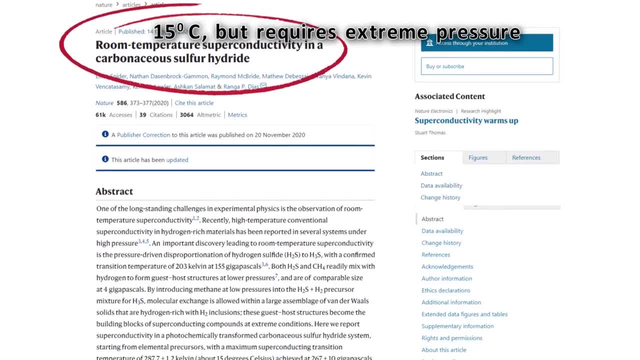 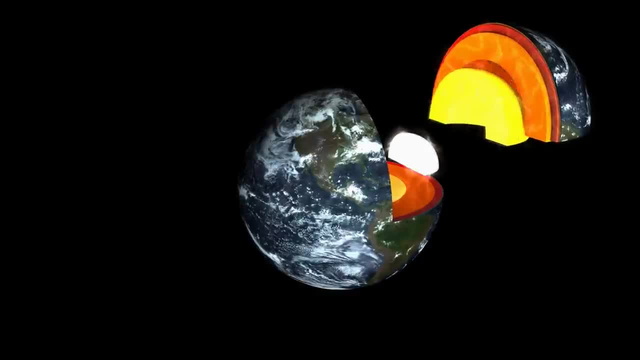 sulfur hydride. Its critical temperature is 15 degrees Celsius or 59 degrees Fahrenheit. This sounds wonderful, but the caveat is that it requires extreme pressures close to that of the center of the earth to work, So it is not quite useful for practical. 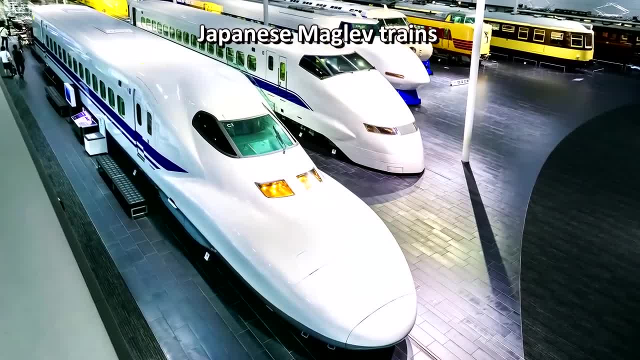 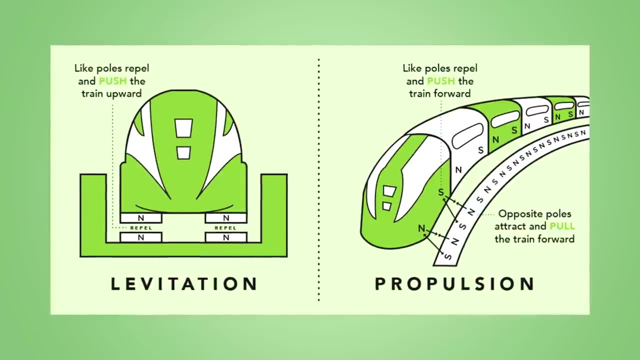 applications, But one really very useful current application is in Meglev trains. In Meglev, superconducting magnets suspend at a very low temperature. This means that superconducting magnets are able to magnetize a train car above a U-shaped concrete guideway And just like.